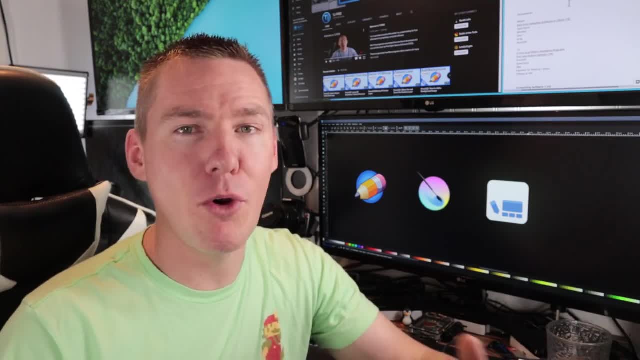 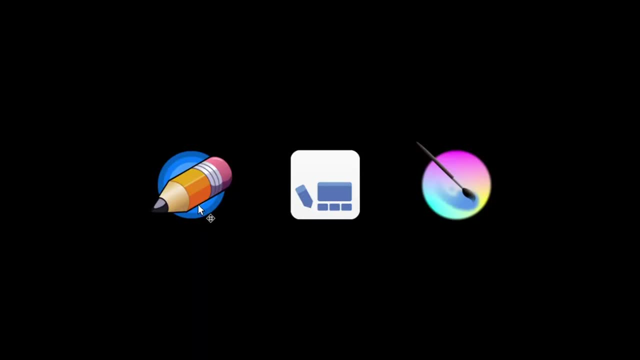 them. I have tutorials teaching these here on this channel. You can learn more about it and polish your skills and learn something you don't know about them by watching those videos. Let's take a look. This first program is Pencil 2D. It's a free program that runs. 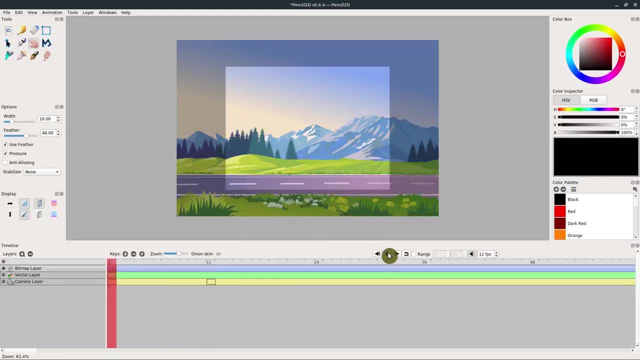 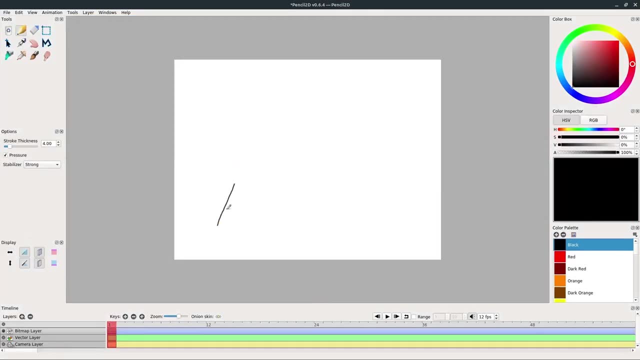 on Windows, Linux and Mac And it has a very simple interface, but it's still very powerful. It sort of reminds me of Microsoft Paint with a timeline built in the bottom. So you have different draw tools, You can draw freehand and you can animate each frame. 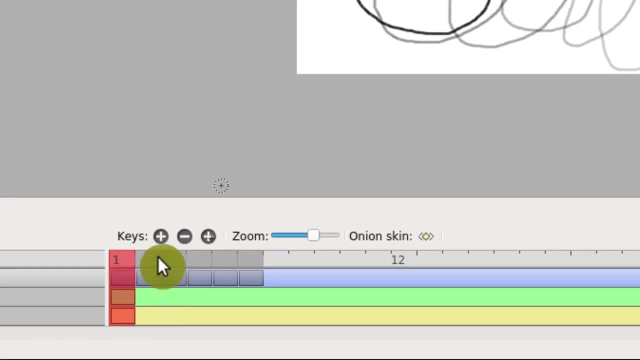 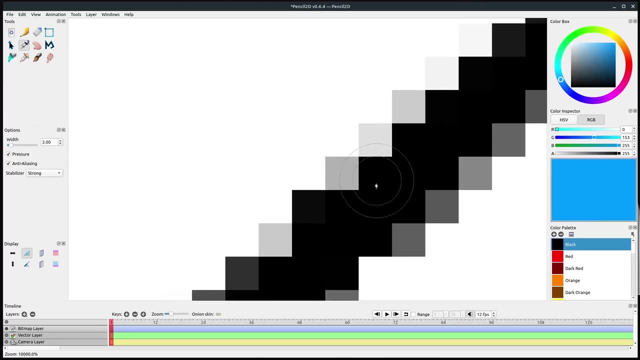 And export it as a video or individual images. You have good control over multiple layers and multiple frames And you can even control the camera- what part of the scene is being viewed. You can zoom in and out, You can work in raster and vector, but it's sort of more. 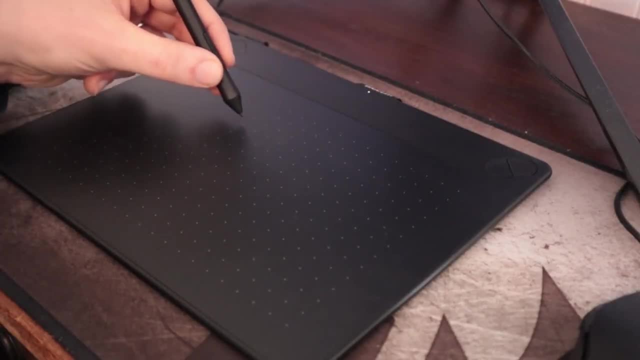 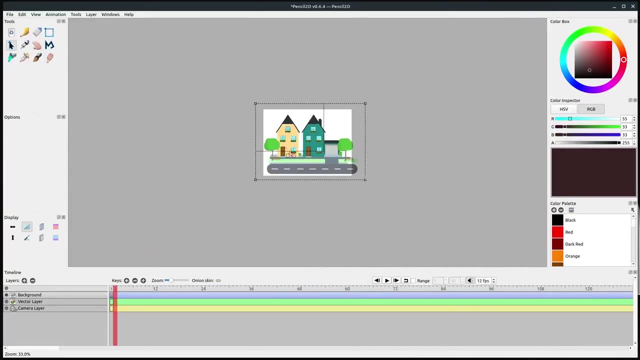 geared towards working with raster or bitmap images. It has good integration for using a drawing tablet if you want to create artwork that way, You can bring in your own artwork as well, or you can download artwork from the internet So you can have multiple layers. 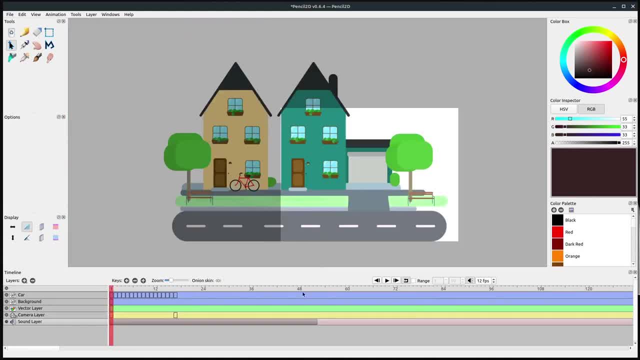 to animate and move that layer each time. So in this case we bring in a car, We just move it frame by frame. Nothing was actually drawn in this. Instead, we just imported the artwork and then animated just that artwork separately. Pencil 2D is very easy to use. 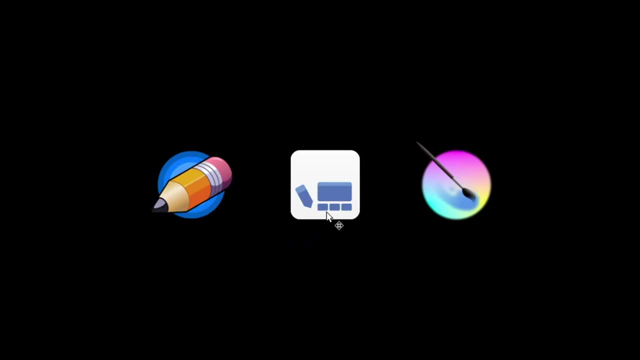 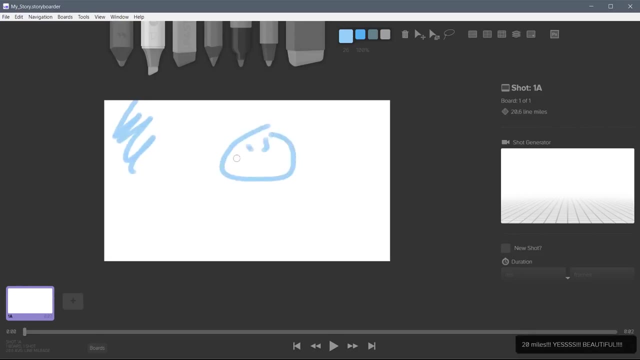 and a great program if you're just getting started with 2D animation. This next program is Storyboarder And it's mainly geared towards creating a storyboard, But it has such good drawing tools and such a nice, clean, easy to use interface. I really 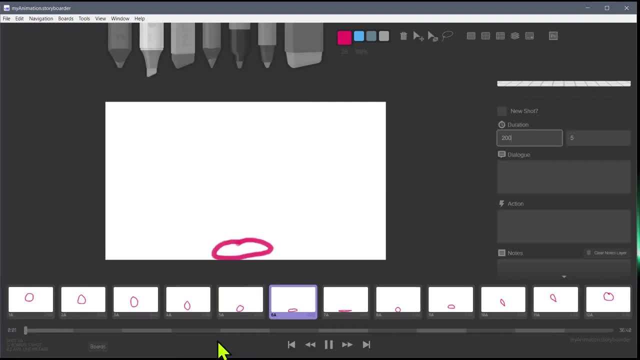 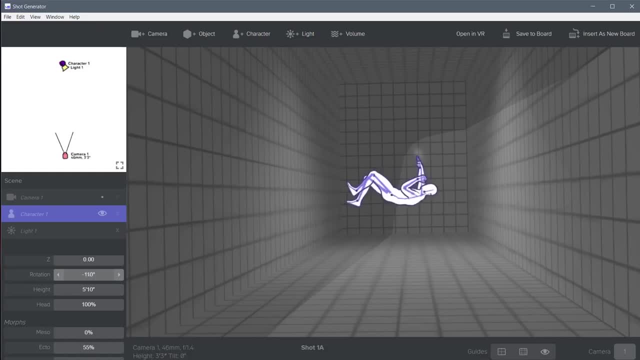 wanted to include it in this video. It does have the ability to work with different boards And you can do some simple animation. You can control the playback of those. But it also has a nice built in 3D engine. If you want to do a 2D animation but with some 3D aspects, It has this really good built. 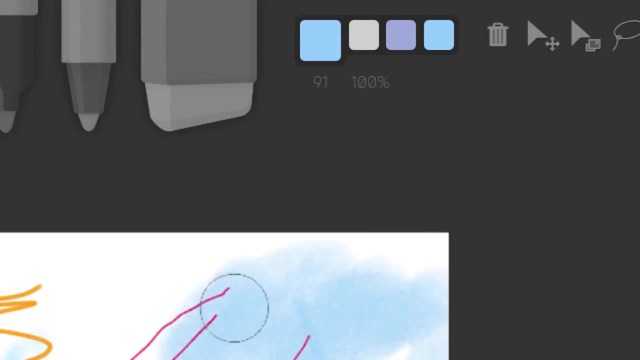 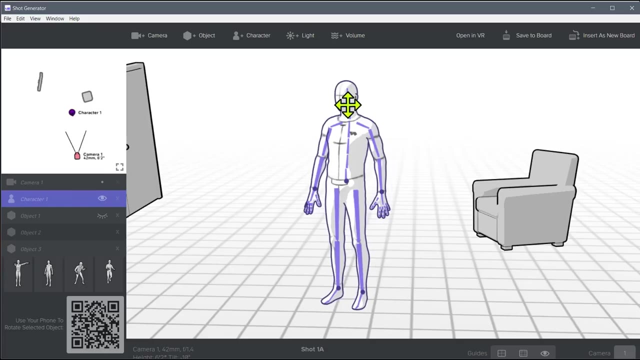 in 3D tool as well. The drawing tools are very nice and well organized. This is a great powerful program, but it's also one that I feel like you could put a student or a child in front of, and they would just intuitively know how to use it. 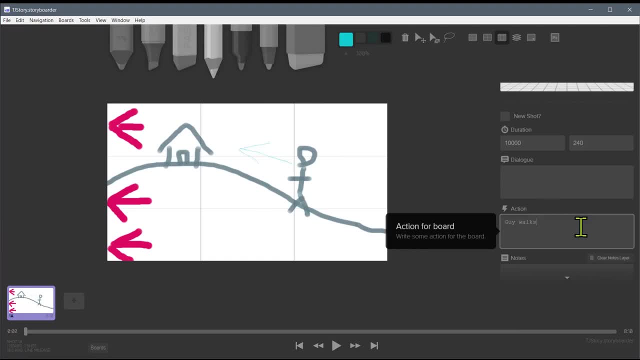 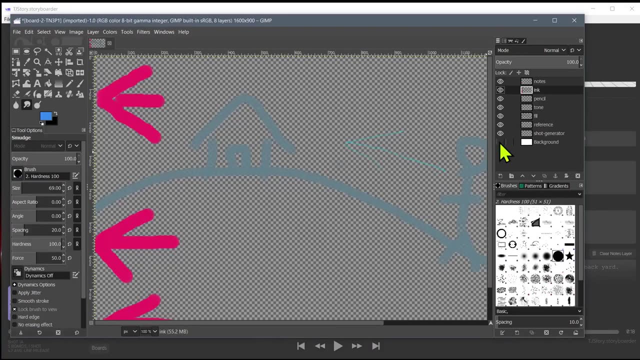 There's not a lot of training involved because everything is very visual: All the different tools and brushes and things that you would do. It's very clear how you would use it. You can also export the artwork to edit in external programs like Gimp or Photoshop.